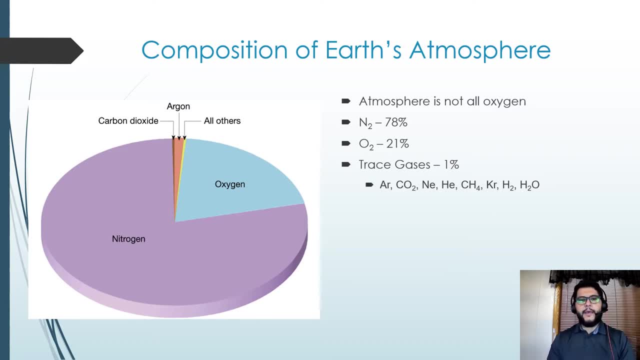 made up of just oxygen. So that's kind of a common misconception. Everybody thinks that, oh, all they're breathing in is oxygen and there's nothing else out there. But actually when you take most of your breath, what you're taking in is mainly nitrogen, So nitrogen tends 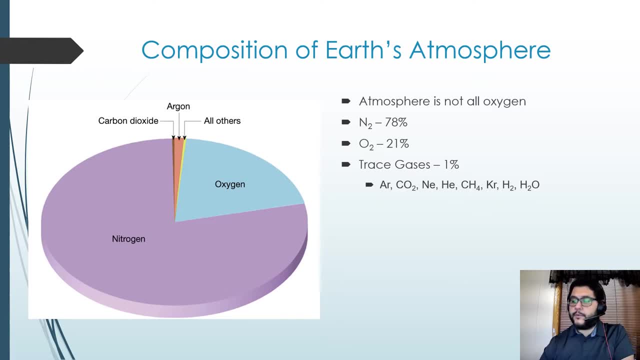 to be the main gas that we're breathing in, and that's going to be 78% of what we have, whereas our oxygen is going to be about 21%. And then the rest is going to be trace gases, and this is the order that you're going to see them in. Argon is actually the next. 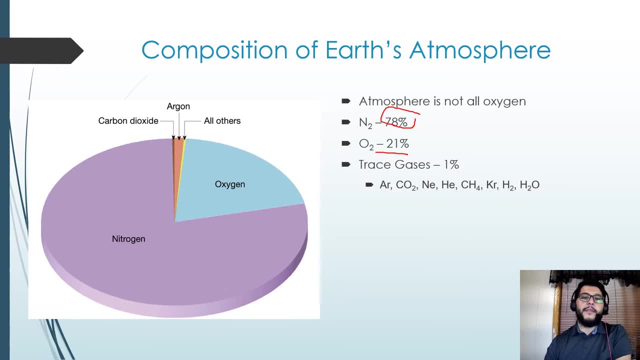 most abundant one. Then you have CO2, neon, helium, methane, krypton, hydrogen gas and water in the atmosphere as well, And so the things to remember about the layers of the atmosphere is: these are all the different ones. 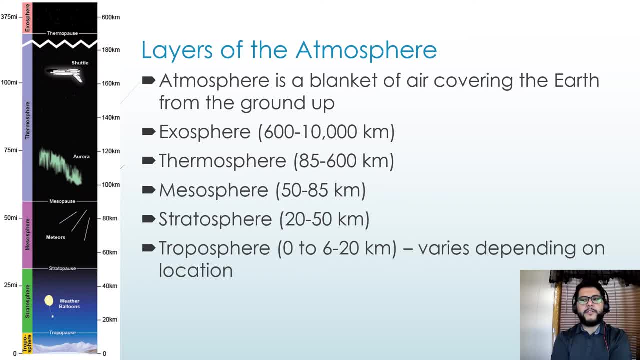 and they're different heights and temperatures. But, honestly, the two layers that I would say you have to be the most familiar with tend to be your troposphere, which is where we are currently So down here, where you have that weather balloon and us, these two layers are going to be the most. 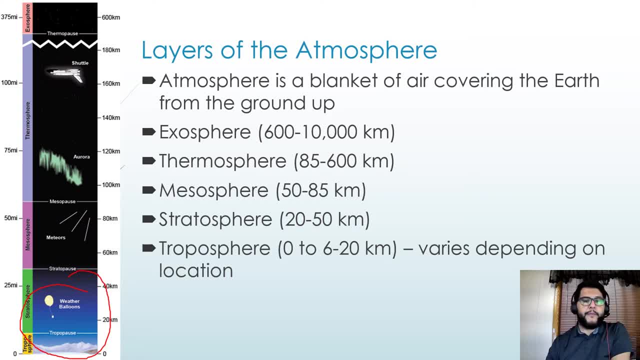 important. That's going to be your troposphere and your stratosphere. You're going to hear that quite a bit later on in the topics with air pollution and ozone are going to be your two main ones, but now it is important still to think about and know these. 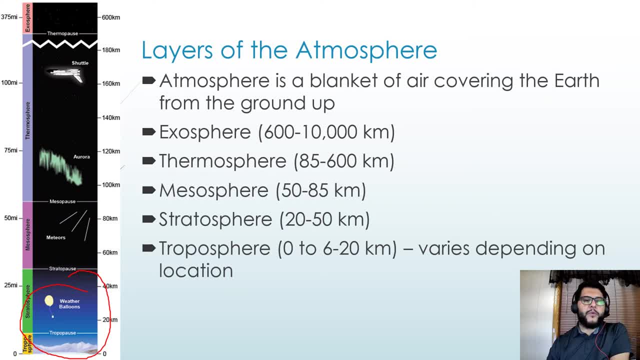 other ones and where they go and what occurs in each one of them. and one of the things that does happen there is there is going to be a change in temperature as you move through these layers, but, honestly, the two most important ones are going to be those bottom layers, the troposphere, and 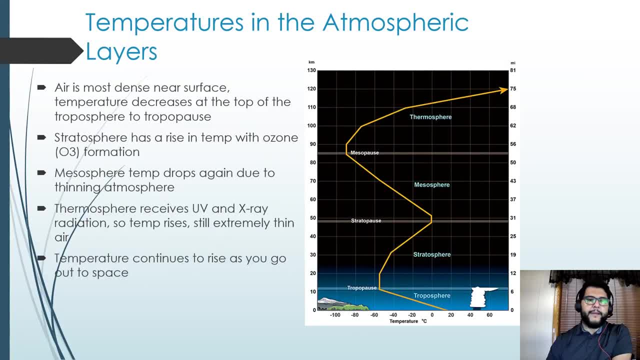 the stratosphere, excuse me. and then right here, as you can see, the air is going to be really dense, um, at the bottom, where we are, and then it's going to change in density. it's going to get much less dense as you go further up and, of course, you're going to have temperature changes. so you're going. 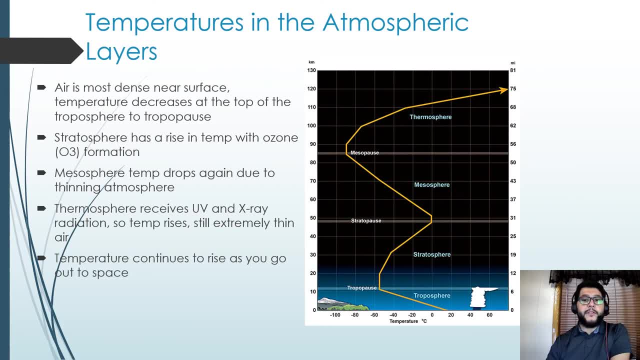 to have a drop in temperature as you go up, then it's going to be a slight rise, and another drop and a rise, and so it's important to note these and see what's happening and why. but, as i mentioned in the previous slide, the two most important ones to be familiar with are going to be down here on the